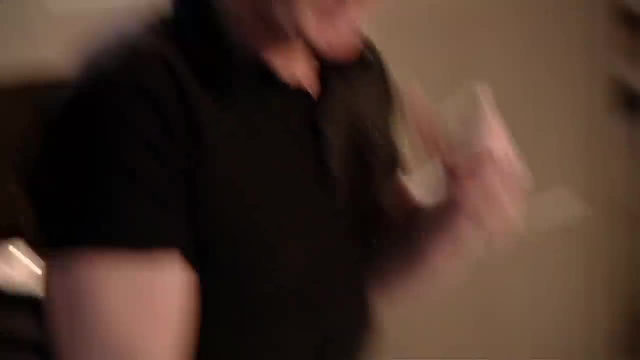 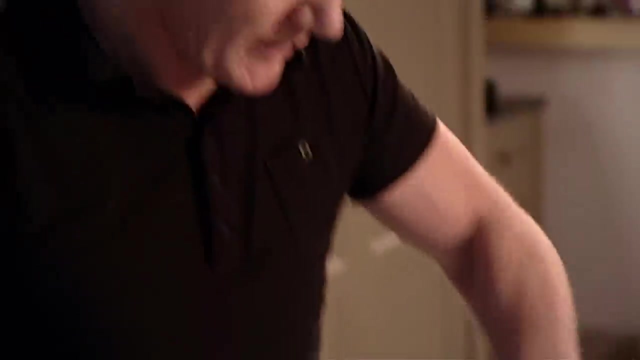 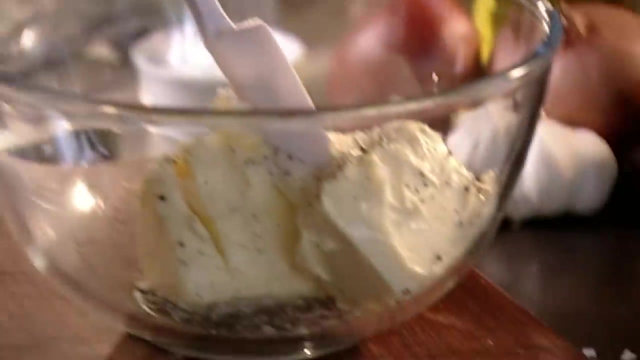 Now we're going to make an amazing butter, and this is sort of the start of the most important part: keeping that bird incredibly moist. Soft butter, a touch of salt and pepper, a little touch of olive oil in there, That stops the butter from burning. 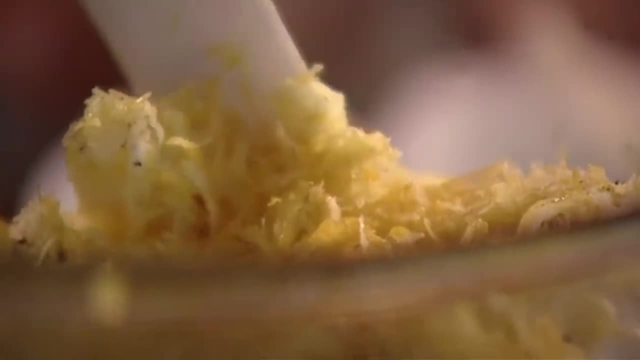 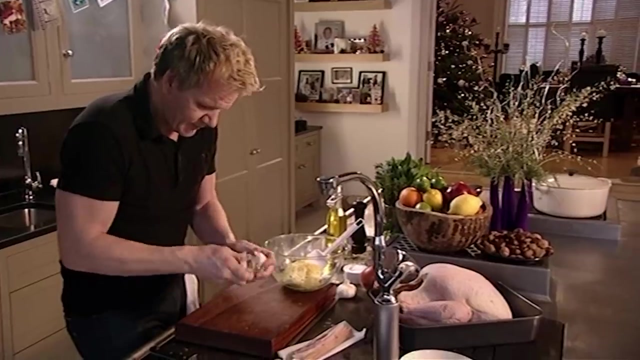 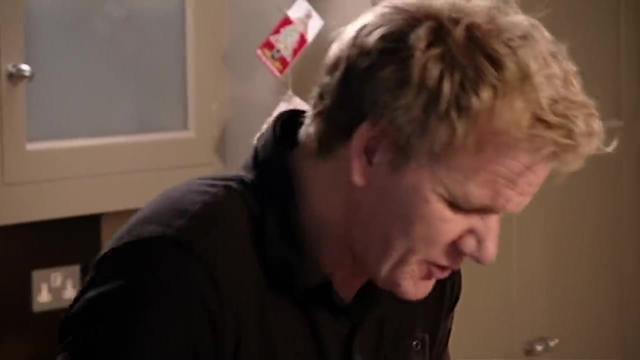 Next add the zest of two lemons and their juice. This gives the flavour of butter, a wonderful citrus zing. Three cloves of garlic: Turkey's a very delicate, dainty meat and that's why I want the garlic pureed so it sort of disintegrates and flavours the turkey gently, without becoming too overpowering. 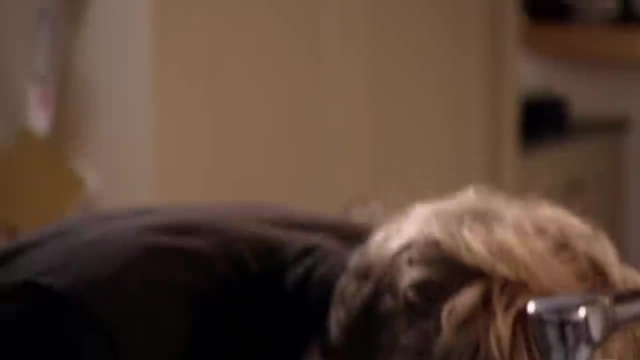 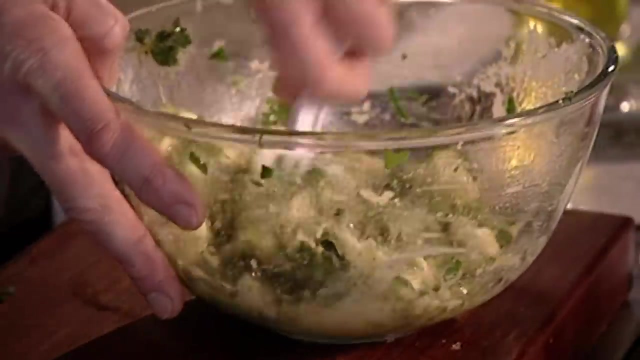 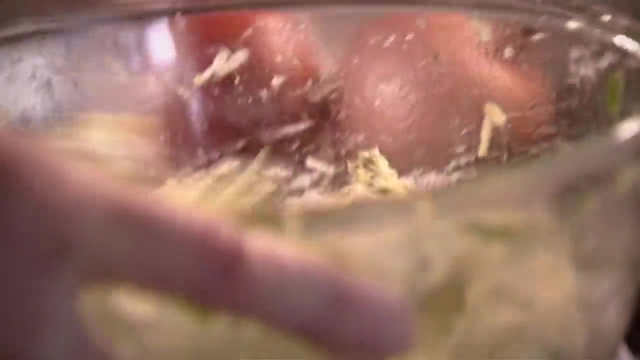 Then add a generous handful of chopped parsley. Wow, that smells incredibly light. Give that a good mix. Turkey's a very, very, very lean bird and it dries out, so it's so important to make sure that we help it to cook perfectly. 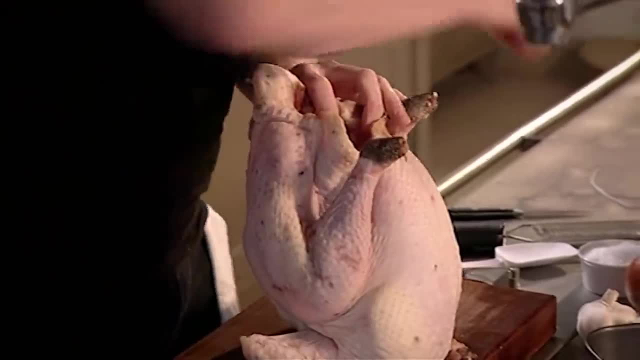 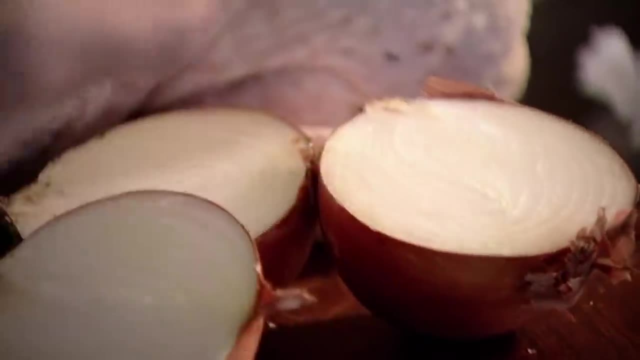 Butter done. Now prepare the turkey. We're going to season the bird Inside the cavity, salt and pepper, Next half two onions and pop them in. As they roast they steam inside the bird, giving it a lovely sweetness. 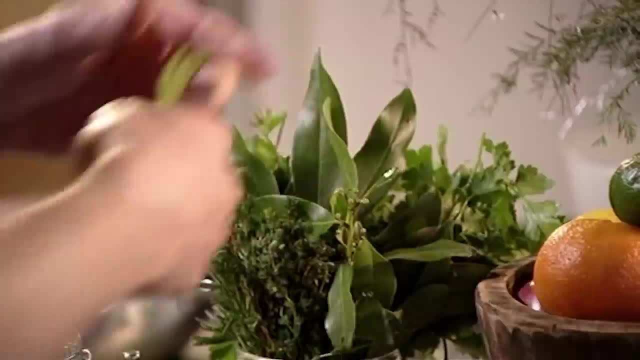 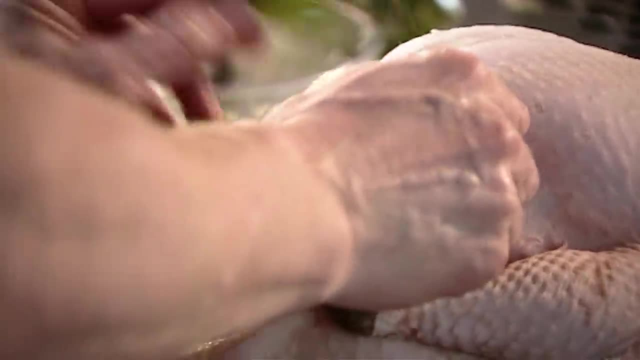 Put in the lemon and a couple of bay leaves for their bittersweet, spicy flavour. We're sort of lining the inside of the turkey with these fantastic sort of flavours. You can see the bird is upright and it's looking sort of like it's standing to attention. 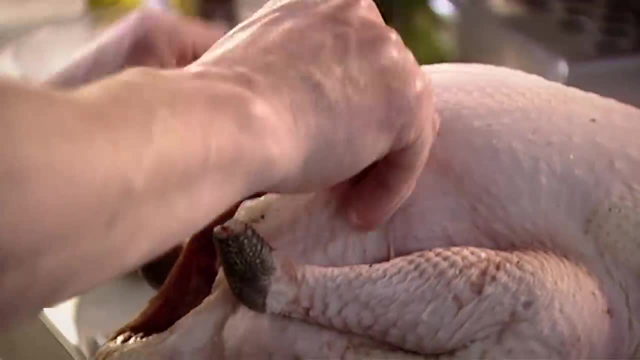 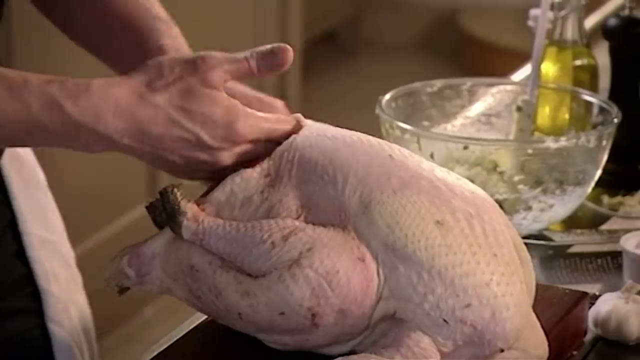 Now it's time to add the flavoured butter. Just, very, very carefully, open up the skin, Go through over the back of the breast and keep the skin intact. The idea is to gently loosen the skin with your fingers So the butter can be stuffed underneath it. 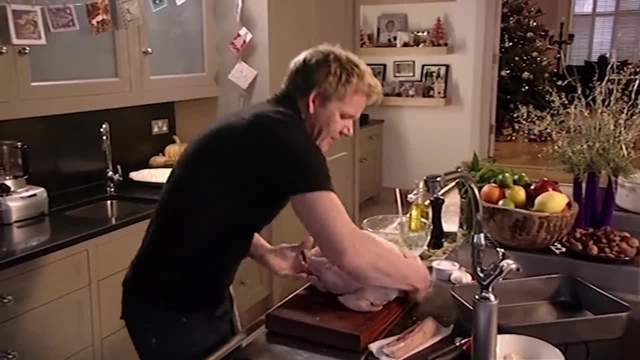 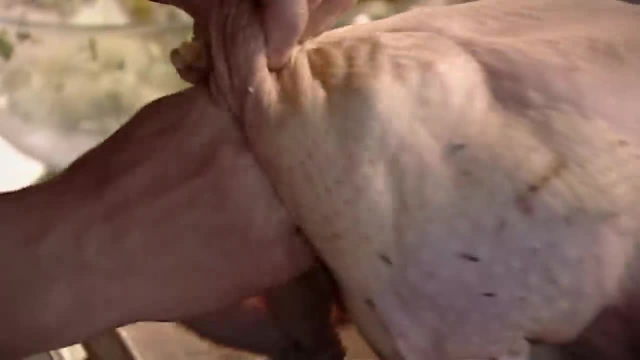 Now, once you've loosened all the skin off the top of the thighs, turn the bird round And just go through here again, Hand up and just release a little bit, But don't completely break it, because I don't want all that butter to run out. 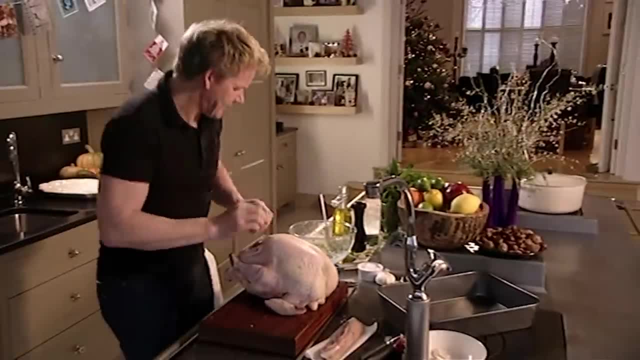 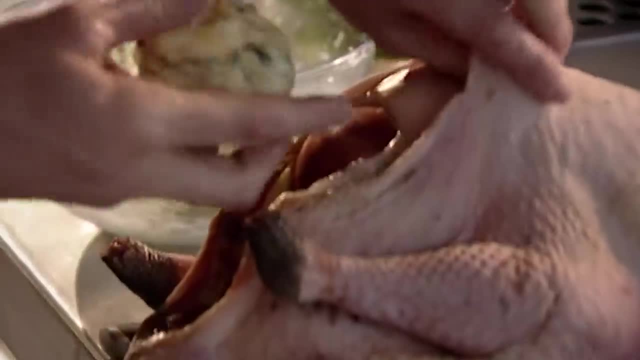 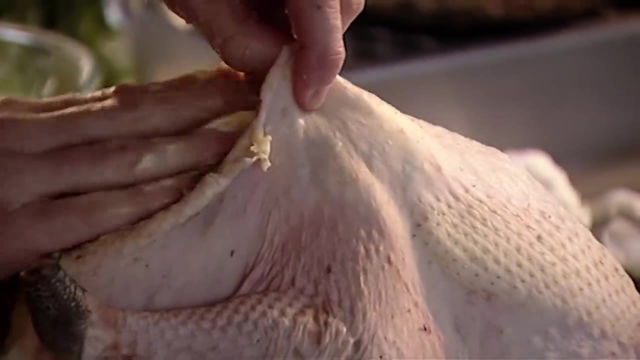 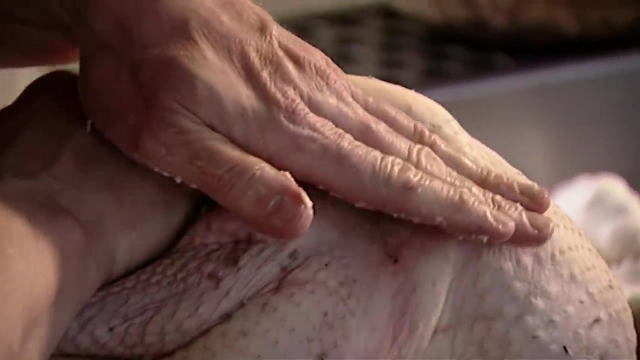 Right from there. Now take your butter, put it into a bowl. It smells amazing: Lemon-y, citrus-y and just sort of fresh. Flatten it and stick that in there Underneath one side. Now, once you've got it in there, pull back the skin and just use that to sort of slide all the way down. 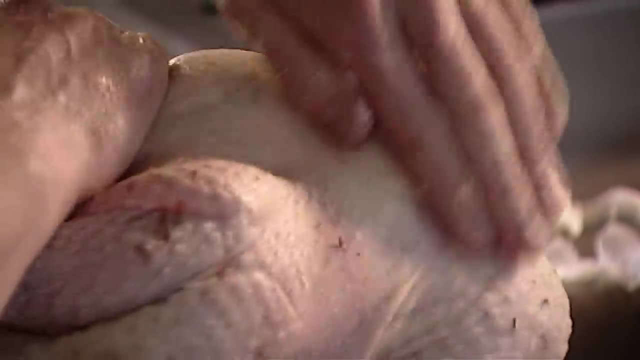 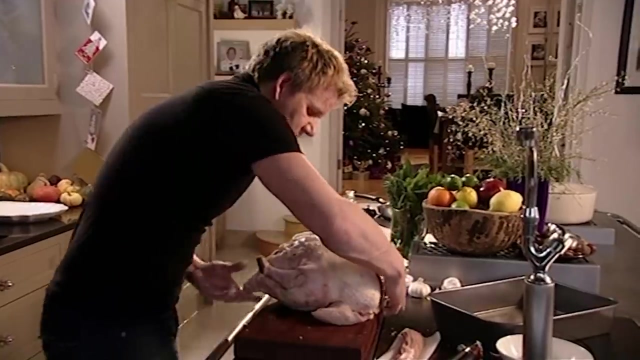 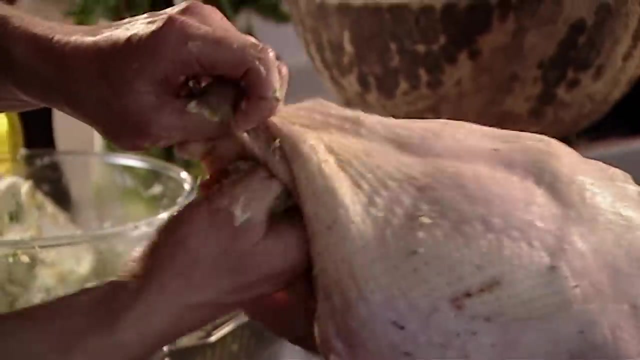 What we want to do now is line the top of the breast with all that butter there. That butter is going to keep the turkey breast really seriously moist. Turn the bird round and finish covering the breast with the butter. Turkeys originally came from North America and they're best young and plump. 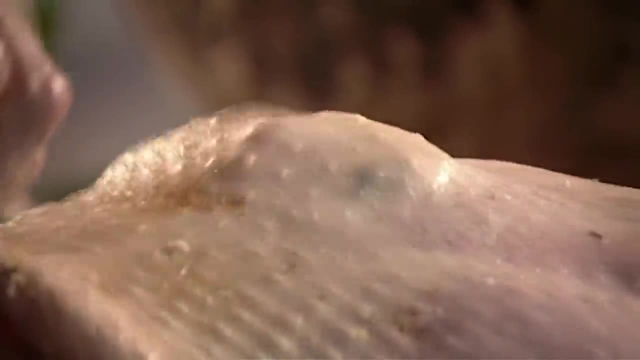 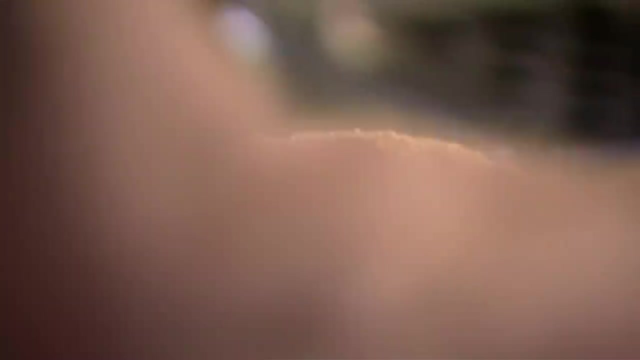 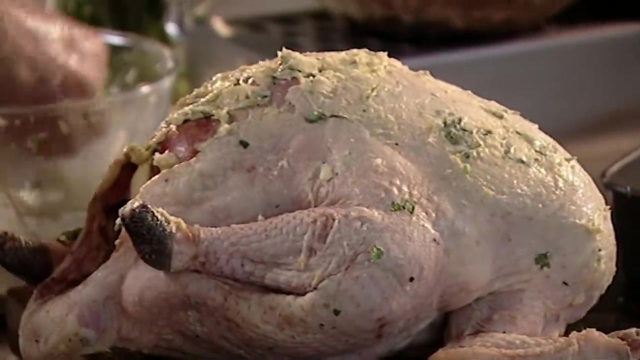 My favourite breed for Christmas is either Norfolk Black or Norfolk Bronze, Both of which have a wonderful gamey taste. Take the rest of the butter and carefully massage over the breast, legs and wings. You can do all this the night before and simply cover the turkey with tinfoil and keep it in the fridge. 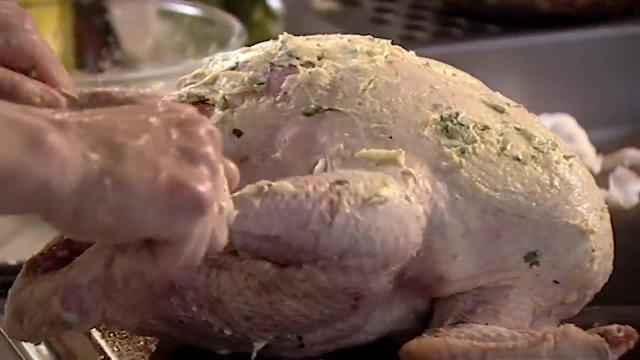 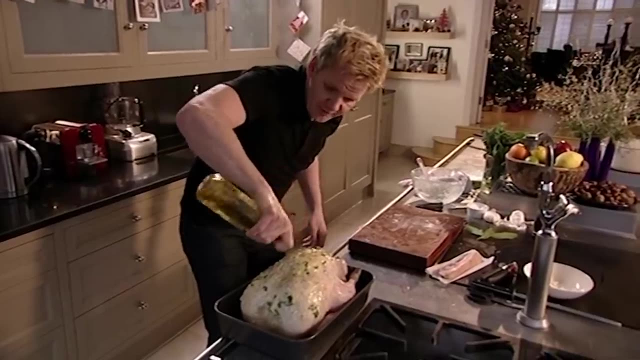 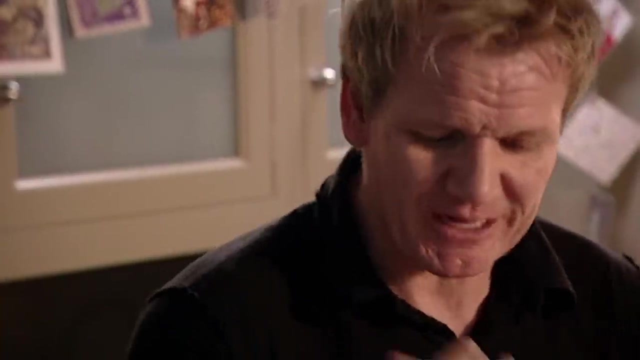 Ready to be cooked on Christmas Day Into the tray. A little touch of olive oil. Now olive oil on top Again. that protects, it Gets that skin really nice and crispy and it stops the butter from burning. Now in the oven at 220 for 10 minutes to get really nice and brown quickly. 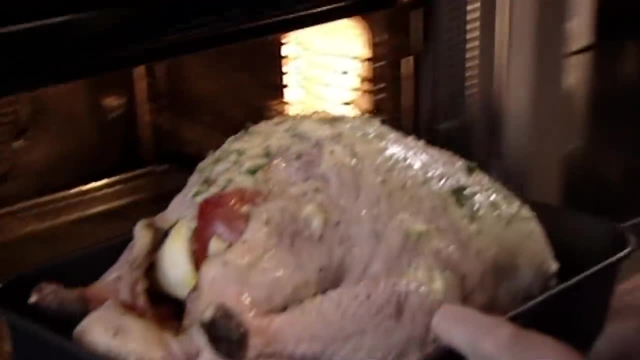 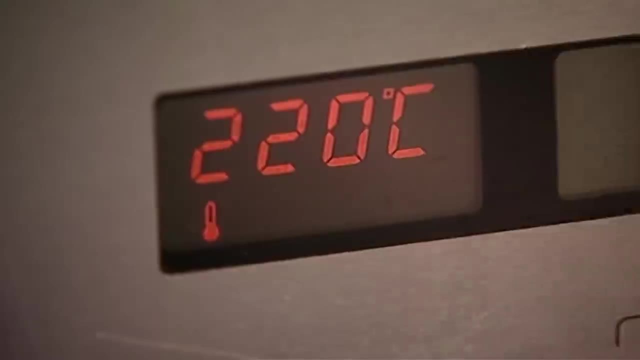 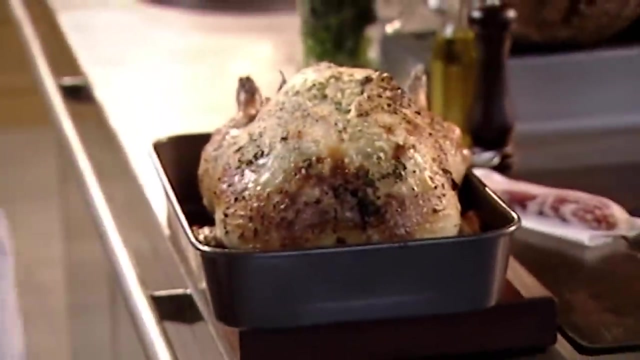 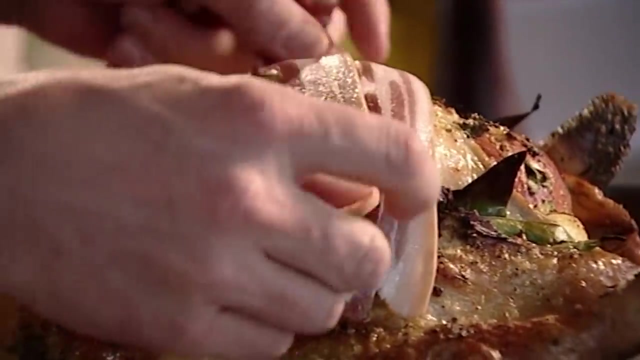 In she goes. Beautiful. That smells fantastic. After 10 minutes, take the turkey out of the oven and baste. Then cover the breast with smoked, streaky bacon. What I want to do is add a little bit more flavour. I'm already starting to think about my gravy. 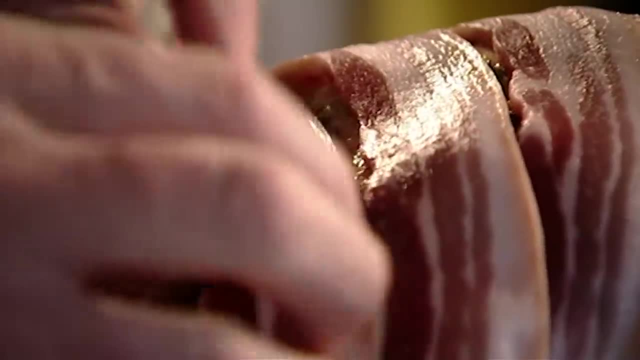 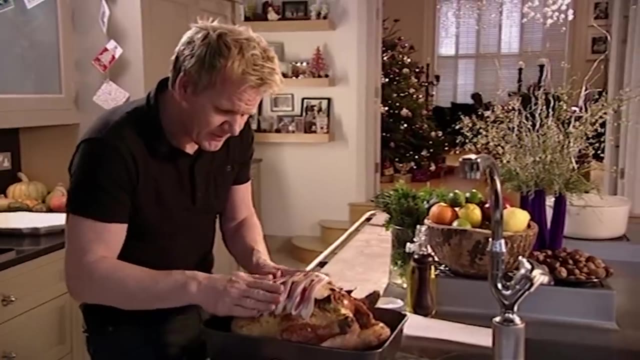 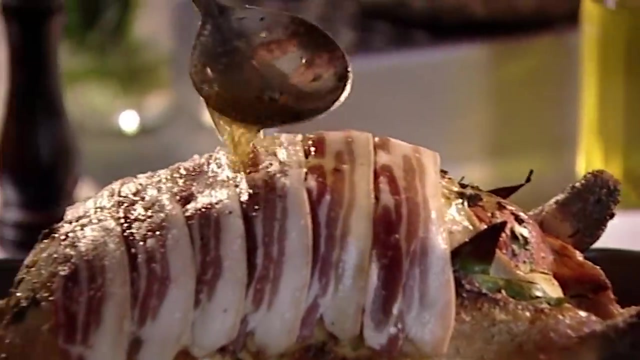 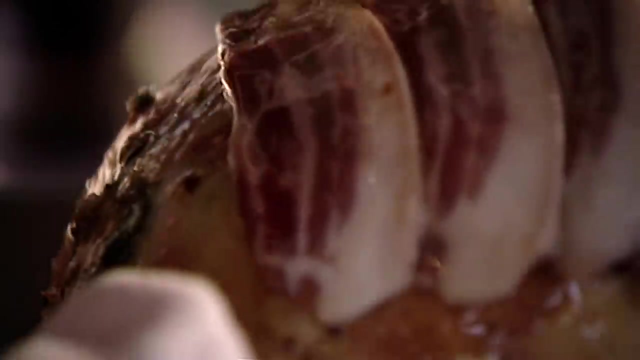 So the bacon protects it, stops it from drying out. but it's going to start to really give my gravy a wonderful base. Turn down the oven to 180 degrees. This five kilogram bird will feed eight people comfortably. It needs roasting for two and a half hours or half an hour per kilo, basting every so often. 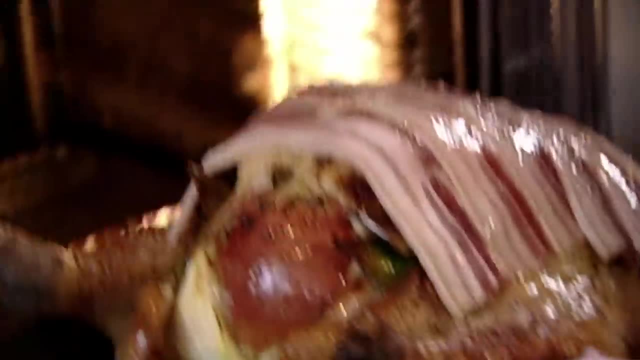 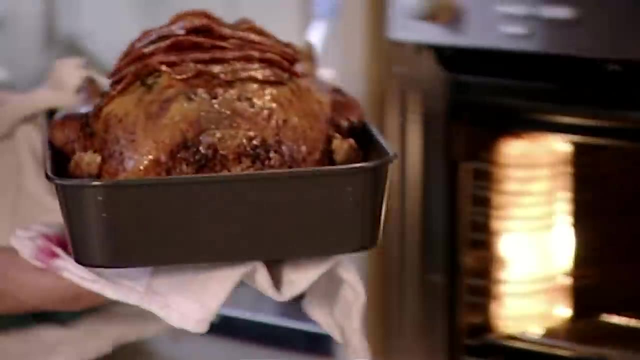 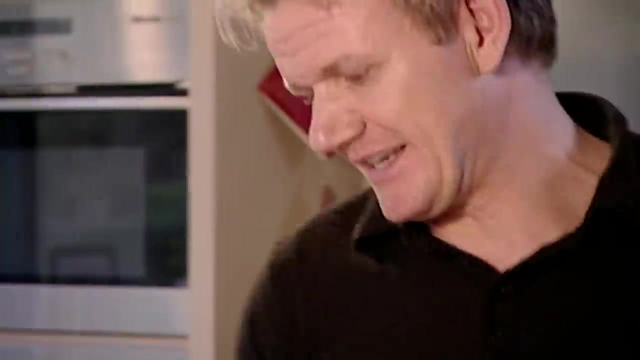 Back in And now she's on the way. Look at that Beautiful. That smells fantastic. Wow, Look at that Beautiful. That is 90% of your work done there. To test the turkey is cooked. stick a knife into the bottom of the thigh. 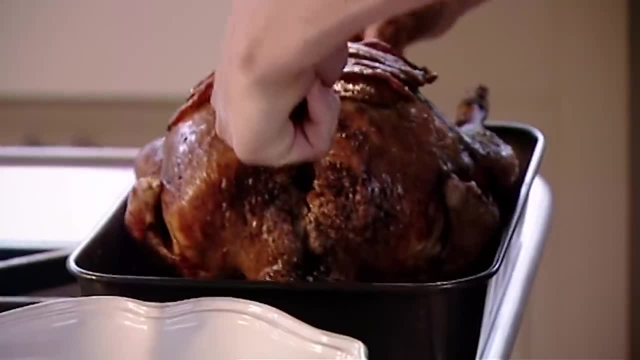 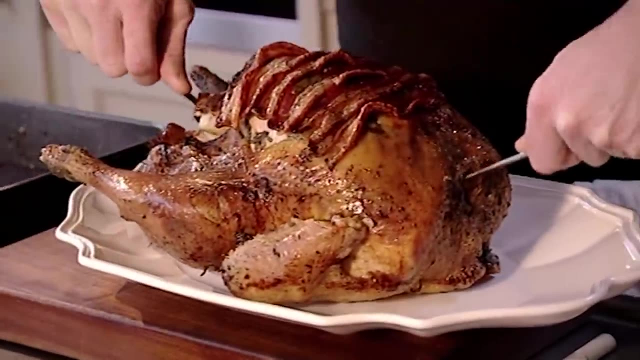 and if the juices run clear, it's done. The secret now is to let the turkey rest uncovered for two and a half hours. As the meat relaxes, it reabsorbs its juices, making it succulent and tender. plus, it will be easier to carve. 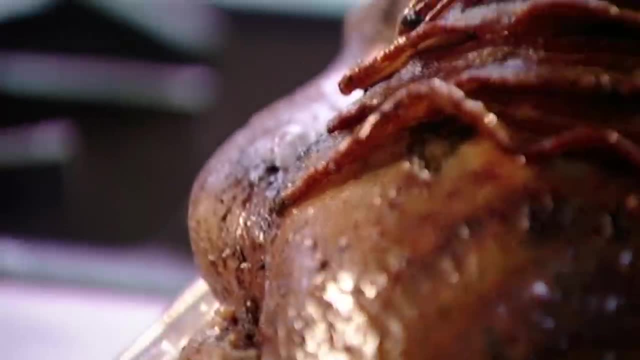 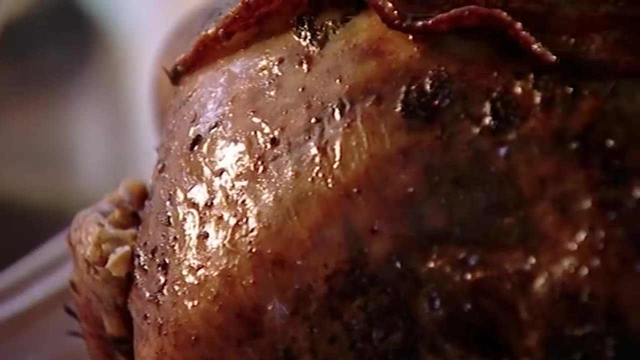 It might seem like a long time to let it rest, but remember, the turkey doesn't need to be piping hot because I'm serving it with hot gravy That looks like a million dollars. Let that rest, because the flavour will be ten times more exciting once it's rested. 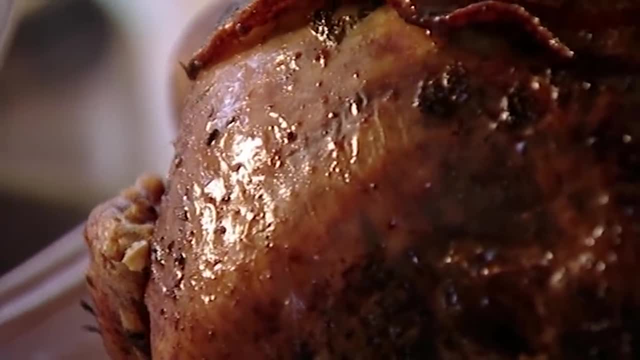 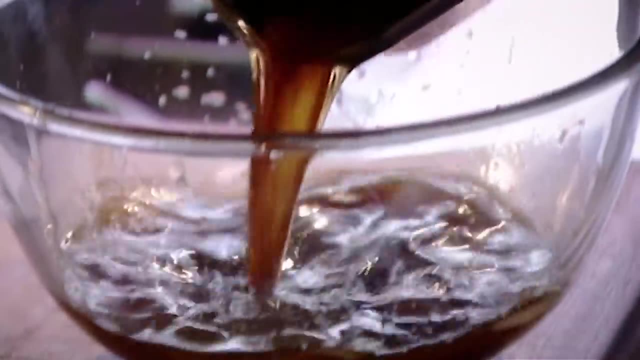 As that turkey's resting, I want to make the most amazing gravy, And when I say amazing, I really do mean amazing. Drain the excess fat from the roasting tray and put it back on the heat, Then remove the bacon from the top of the turkey. 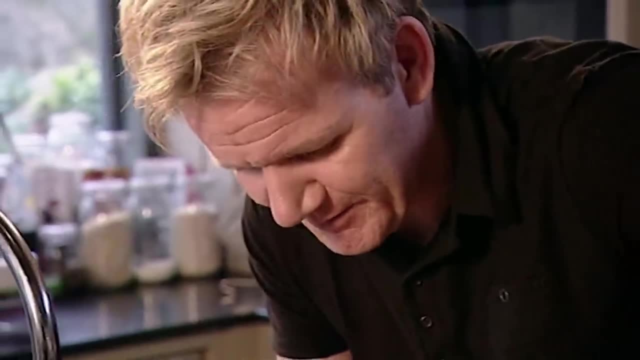 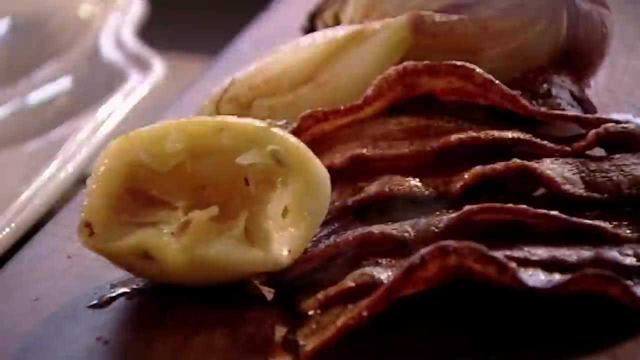 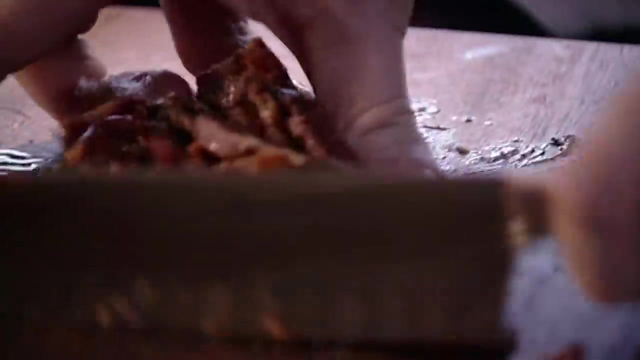 and the roasted onions from the cavity. Look at them, My God, they smell amazing. Finally, take out the roasted lemon. First of all, cut up the bacon- Lovely Bacon- into the tray. Hear how crispy that is. That's the start of our gravy. 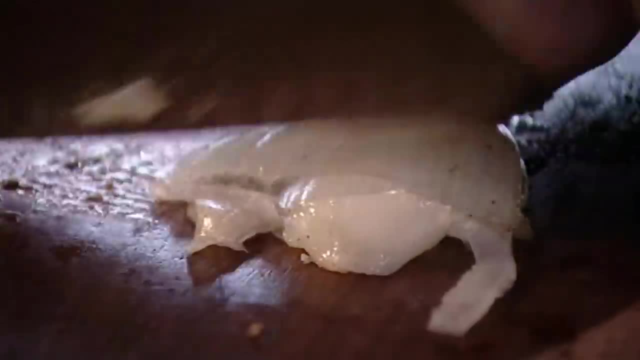 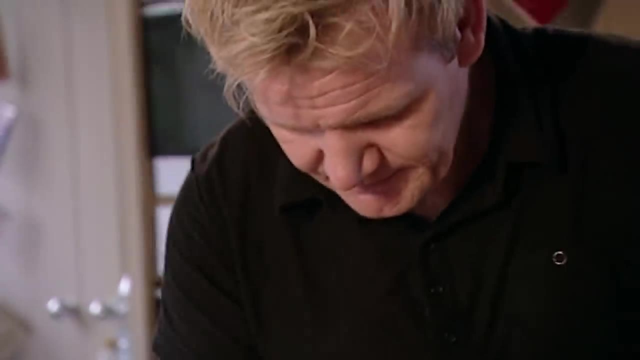 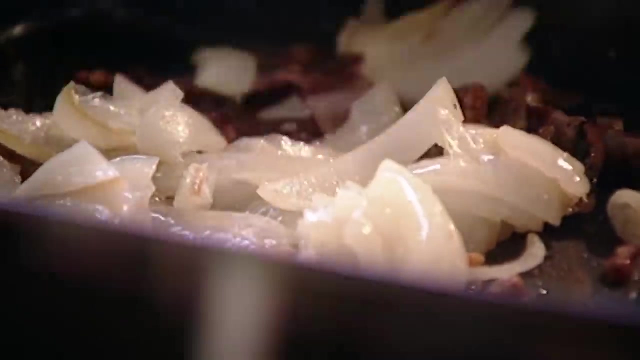 The onion. look at it, Beautiful, Doesn't get any better than that. Chop that up: Onion and bacon in. That smells incredible. When I first got the chance to cook Christmas lunch for the chefs in Paris, they taught me one crucial thing. 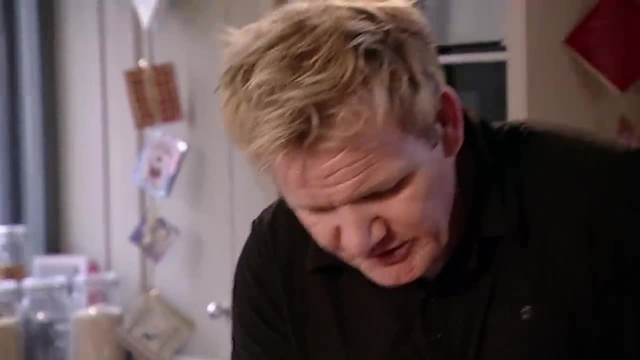 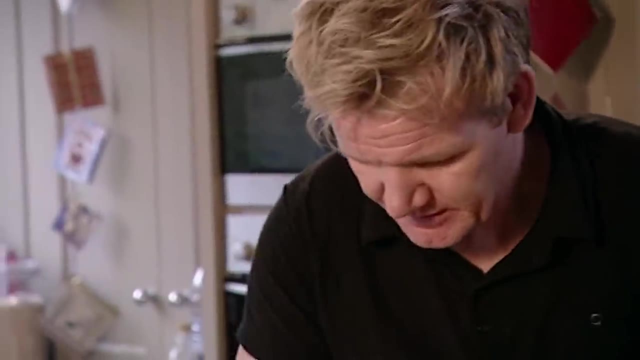 I was only 21 at the time and they made me rest the turkey for as long as I cooked it. So I cooked it for three hours and I rested it for three hours. What a difference, Incredible. Next, chop up the roasted lemon and add to the tray. 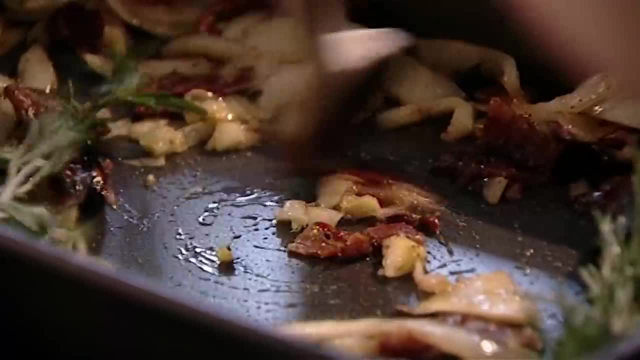 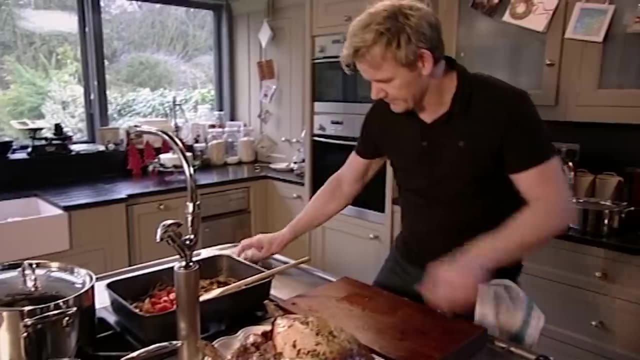 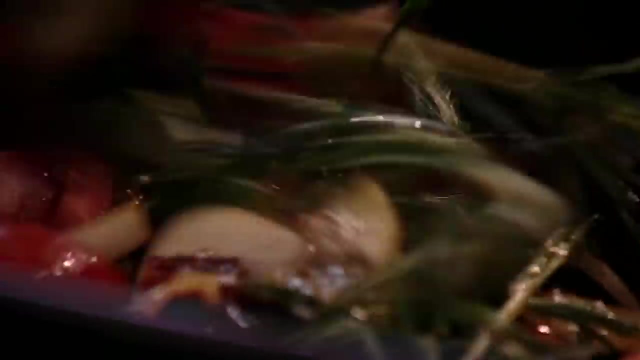 Put in a couple of sprigs of rosemary to give it a lovely aromatic punch, and fry. Then add three chopped tomatoes, which helps to thicken the gravy and give it a lovely fresh taste. Now it's time to really get the turkey flavour into the gravy. 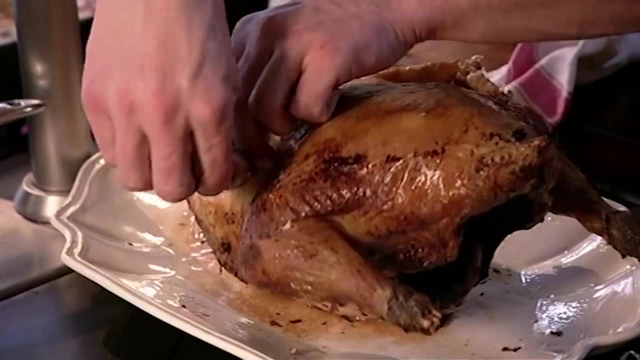 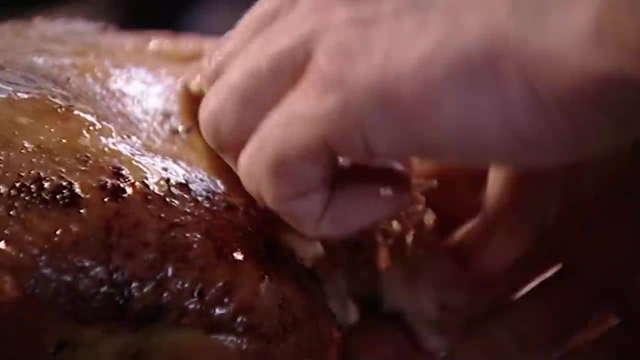 Snap off the wing. Take off all your little trimmings, All these little bits here. Add that into your gravy. These are the bits we never use. Everyone throws them away. Off. There, That little baby there. Take him off. 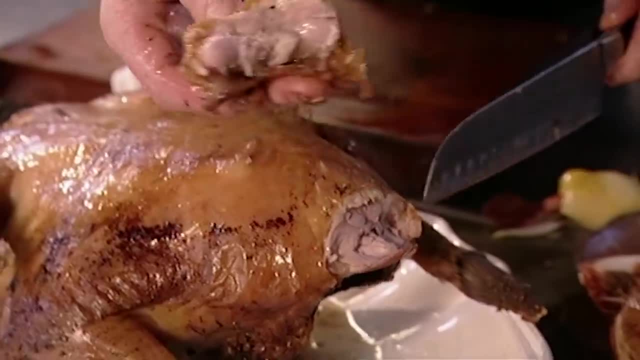 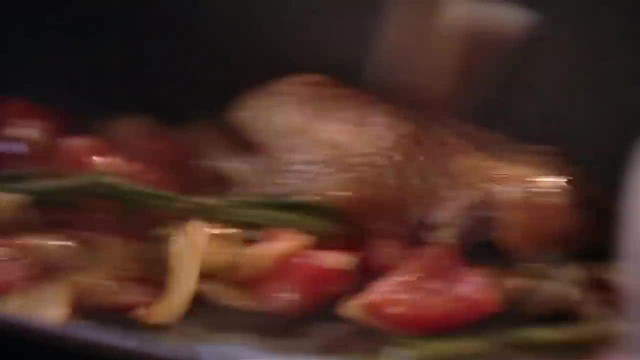 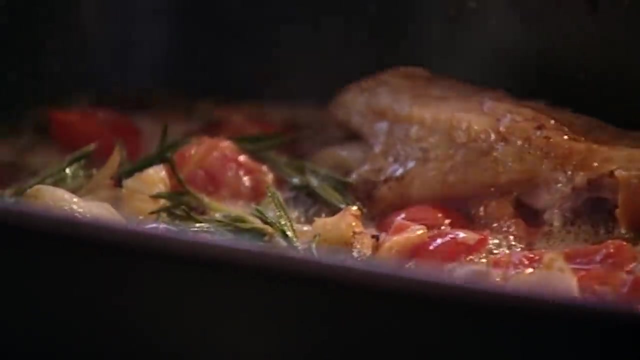 I want that Bang Flavour Delicious. Fry that off. The smell is incredible. Next, pour in the dry cider. This adds a lovely, subtle apple flavour that really lifts the taste of the turkey meat As the cider starts to reduce. 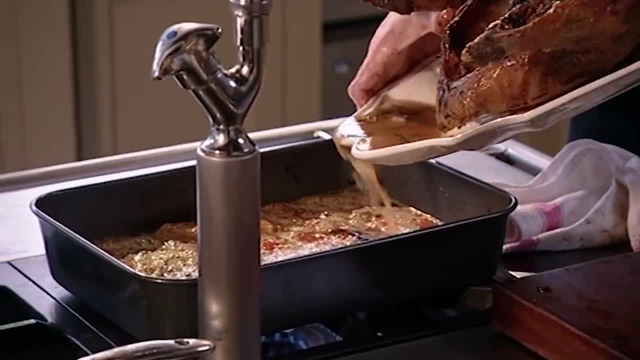 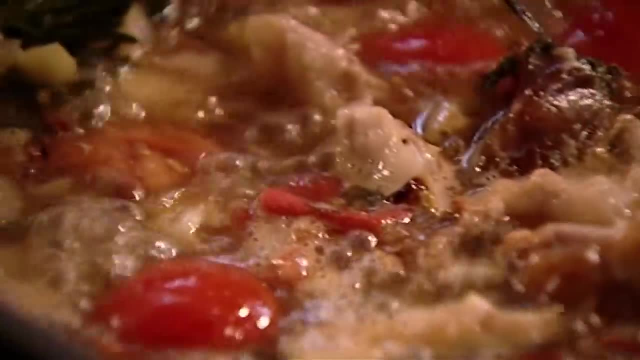 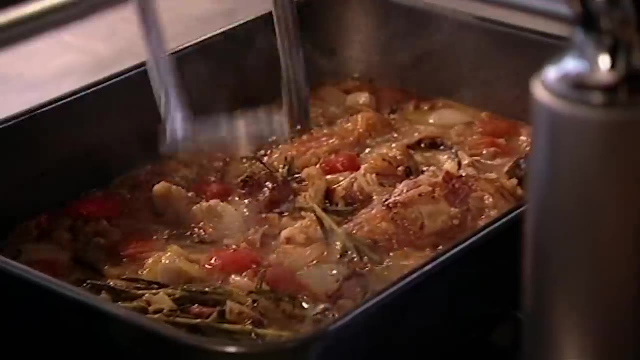 pour in the delicious resting juices from the roasted turkey. Wow, There you go, The most amazing flavour. When the liquid has reduced by half, crush the vegetables and the turkey pieces with a masher to extract the maximum amount of flavour And basically, what's happening now is that we're giving the gravy. 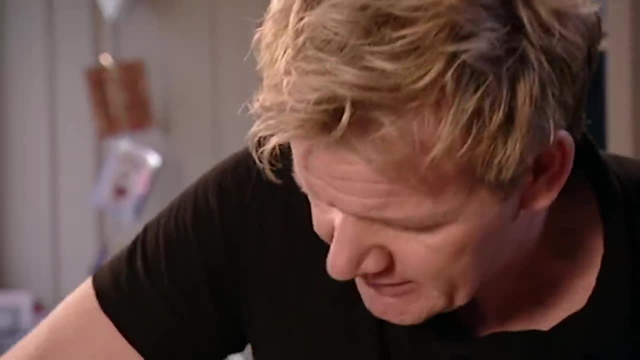 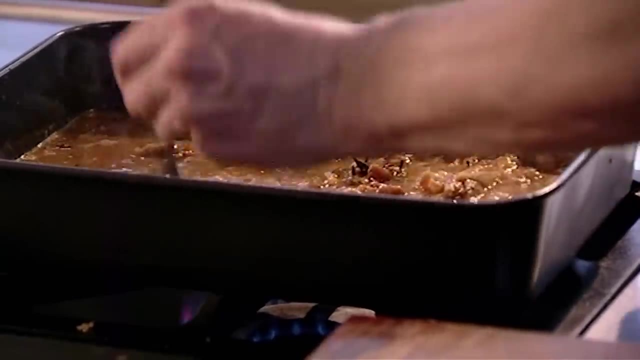 a little bit of body, Pour in the chicken stock and reduce again In. Now a little taste. Wow, I mean, you just close your eyes and wow, it oozes flavour and turkey. Now we're going to add the chicken stock. 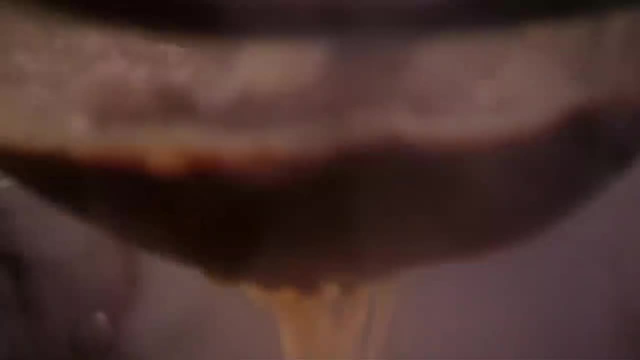 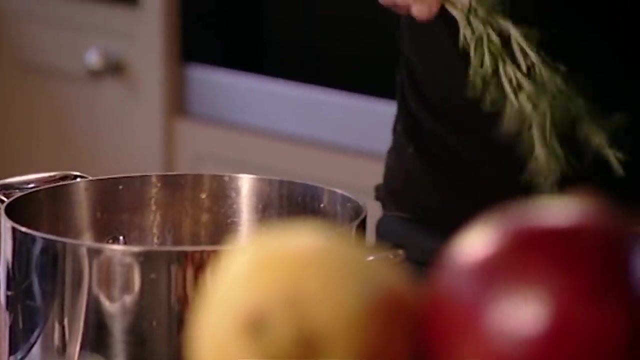 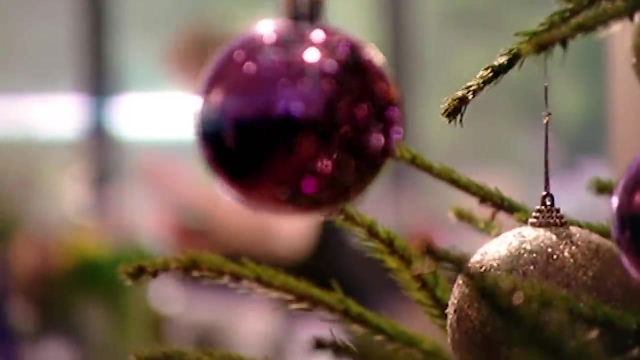 And turkey. Now sieve it. Use the back of the ladle to push it through the sieve, extracting every last drop of flavour. Pop in a sprig of rosemary and leave to infuse. ready for the finishing touch, Simply add crushed walnuts to the bottom of the gravy boat. 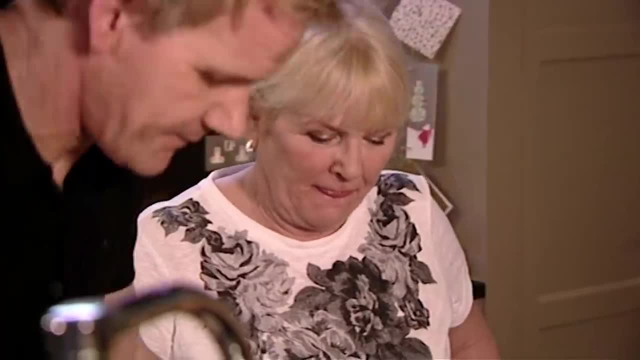 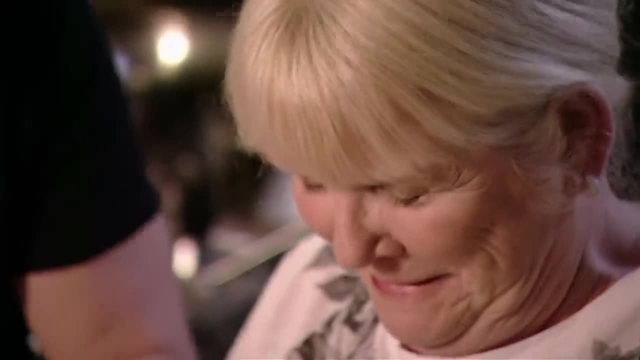 and ladle in the hot gravy. I'm just going to do again a little twist of the potatoes. We do need some goose fat, Harry, No, no, Oh God, Goose fat, And we're going to do a really nice lightly spiced roast potato. 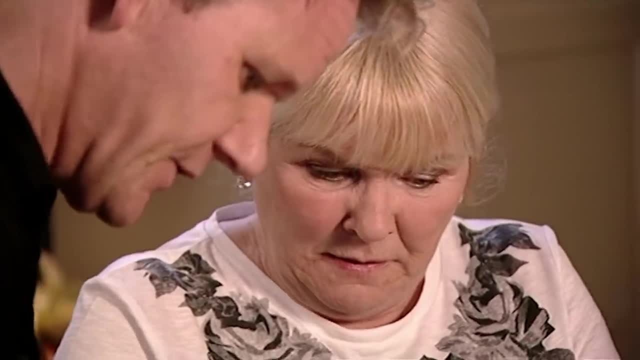 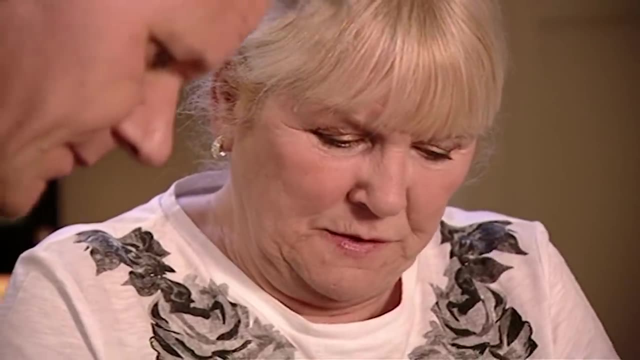 OK, A little chilli flake. Chilli, Yeah, chilli flake. Just put a little bit of heat in there For the Christmas lunch. Yep, Chilli flake and a little bit of turmeric. I can't believe you're doing roast potatoes with chilli. 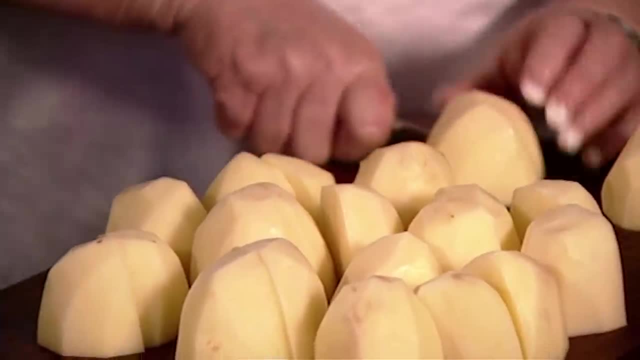 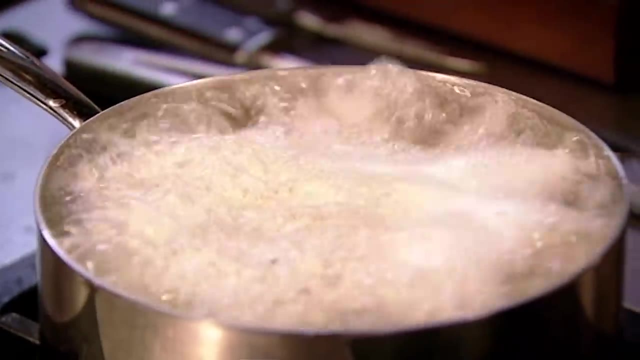 Now would you be so kind just to give them a little cut. Cut the peeled potatoes into quarters and put into salted cold water. In they go, OK. Bring them up to the boil and simmer for around eight minutes, Drain and let them steam. 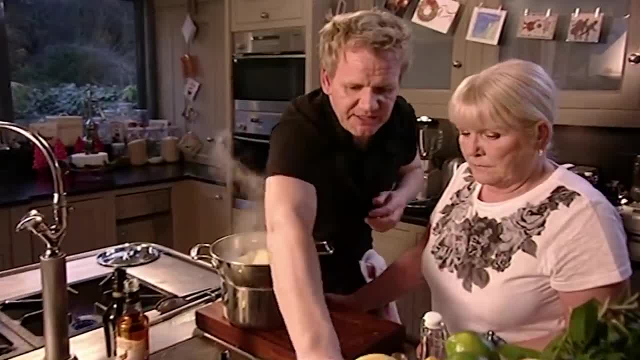 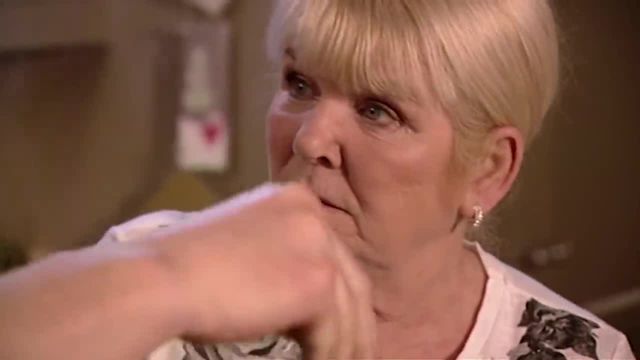 Then season with salt and pepper And just a little teaspoon of chilli flake. Ooh, No, That's the sort of thing I would make for supper on a Saturday night, or something like that. you know, Really Chilli flake's in. 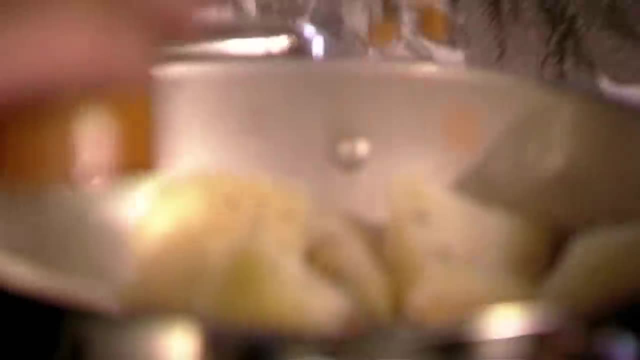 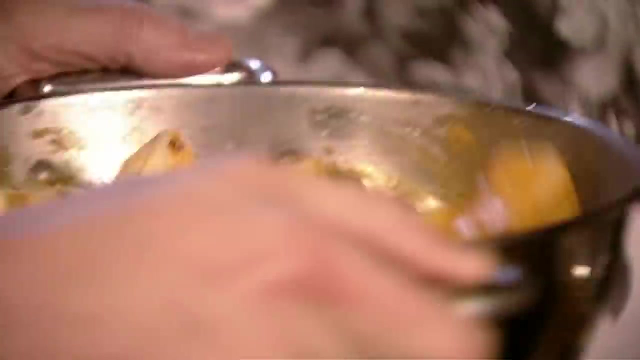 Add a teaspoon of turmeric. Turmeric is a member of the ginger family. It stains the potatoes a wonderful golden colour and adds a lovely earthy taste. Next, drizzle in a little olive oil and shake to coat them. Just let them roll round. 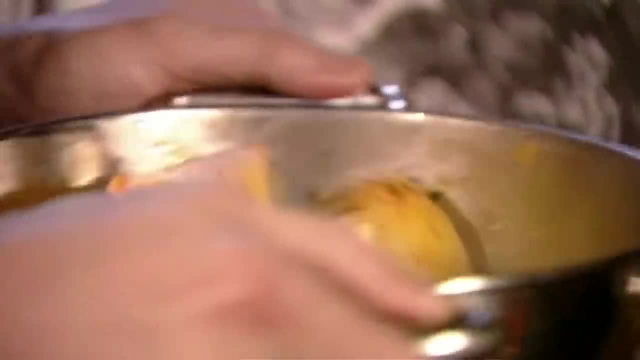 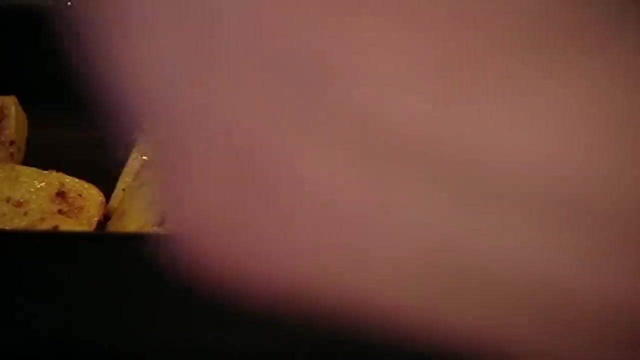 Yeah, That smells nice, Beautiful. Could you get me the stuffing please from the fridge, Put in a preheated baking tray with extra olive oil and cook at 200 degrees Celsius for about 40 minutes. Give them a little shake to make sure they don't stick. 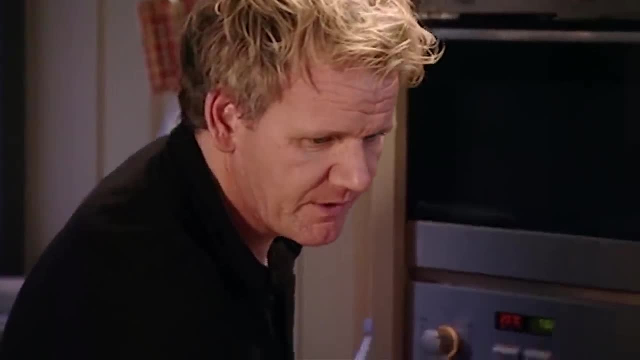 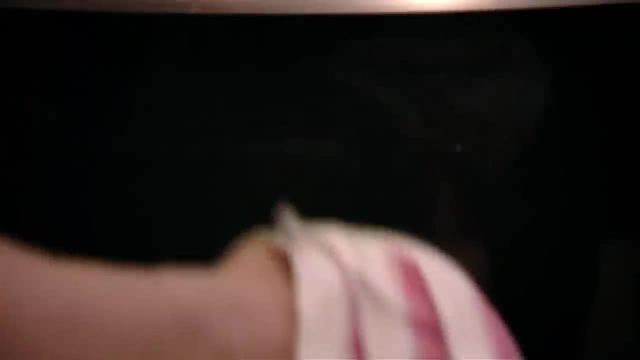 And then I'll just stick the stuffing Hang on on top. yeah, Now, that will take roughly about the same time as the potatoes Stuffing in potatoes done. Nice, Why don't you go play with the kids? 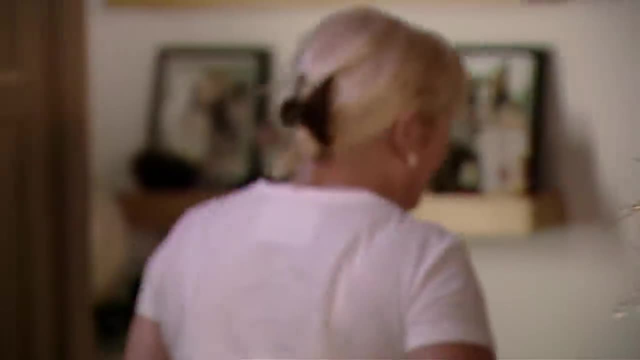 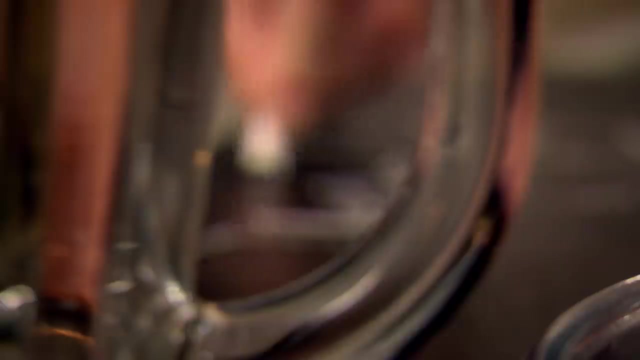 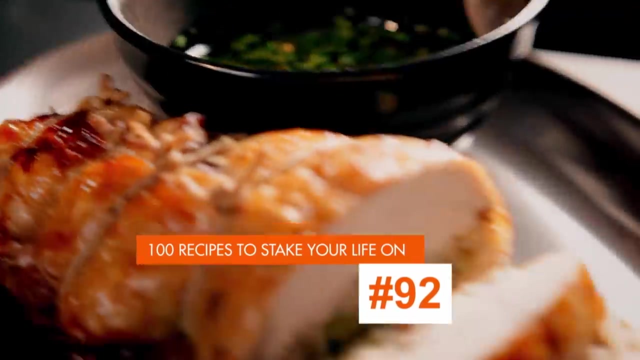 I will do. yeah, OK, see you shortly. Thank you, Bye-bye. Now they look and smell fantastic. Look at that Beautiful Chicken with garlic and chestnut stuffing, packed with flavour and earthy richness For the stuffing fry. finely chopped onion. 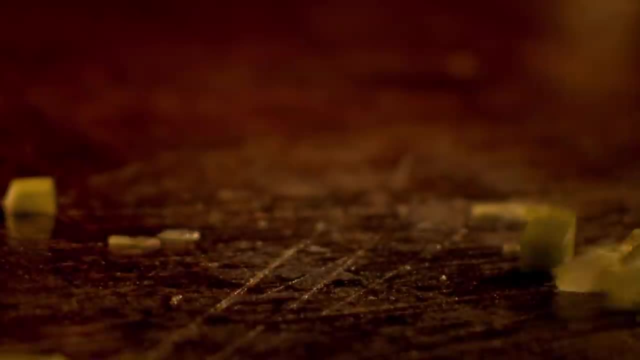 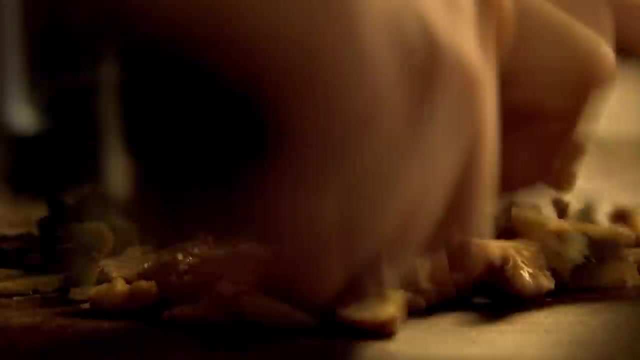 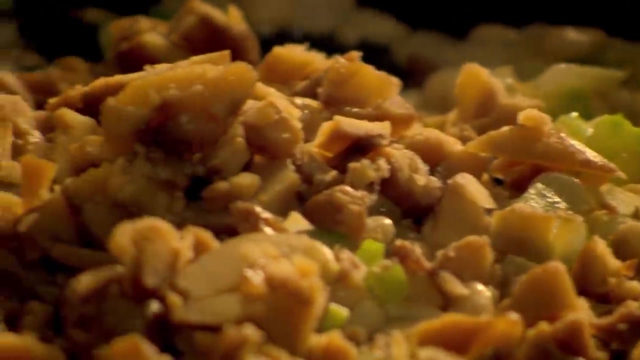 garlic and celery in hot olive oil. Next add pine nuts, which have a lovely creamy taste, and chopped earthy-cooked chestnuts. Both add a wonderfully chewy texture and richness to stuffings Season and add chopped parsley. 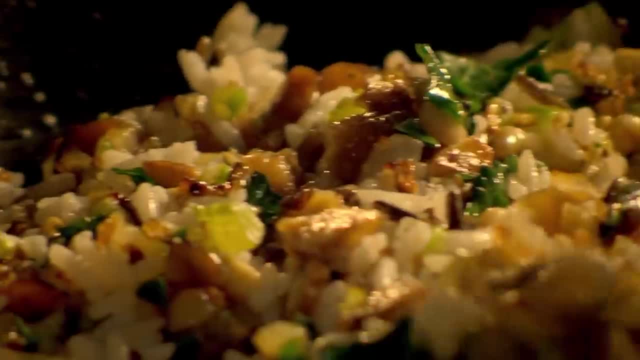 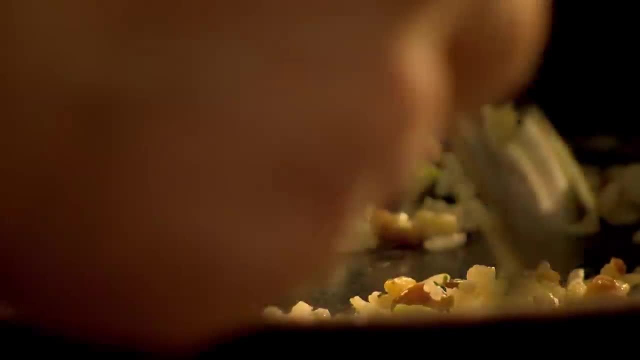 Then stir in cooked wild rice. Next, take a whole deboned chicken- It's fiddly to do at home, but if you ask your butcher will do it for you- And pile the stuffing mixture along the centre. Now simply roll the chicken up tightly. 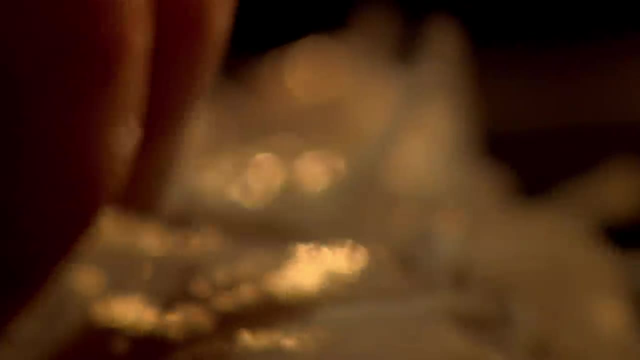 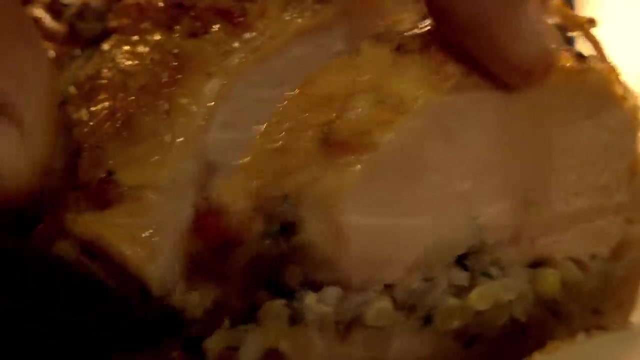 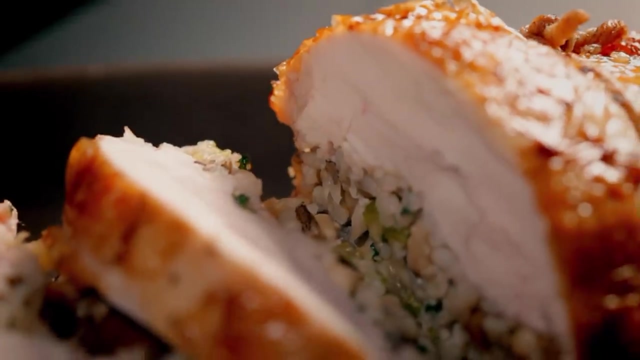 and tie it with your butcher's string, Then roast in a hot oven for just over an hour, Simply carve into magnificent thick slices. So impressive, so easy and, trust me, this is a dish guaranteed to get a fantastic reaction on any occasion. 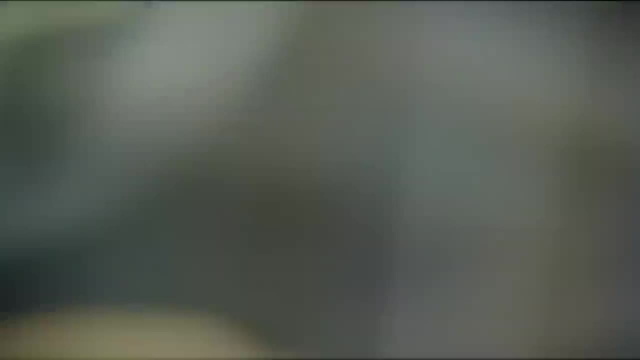 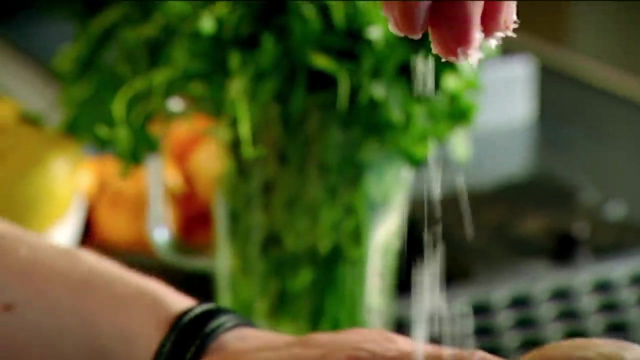 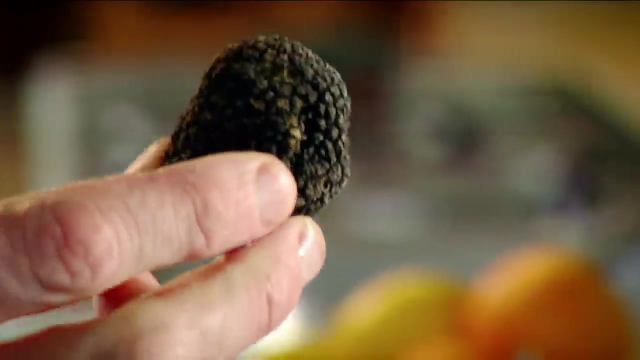 Turkey, The one-hit wonder, An absolutely amazing burger Stuff, Onion, Orange Garlic, Thyme and bay leaf Season Truffle butter. This little beauty helps to take the turkey to a different division. These cost 50 quid for that size. 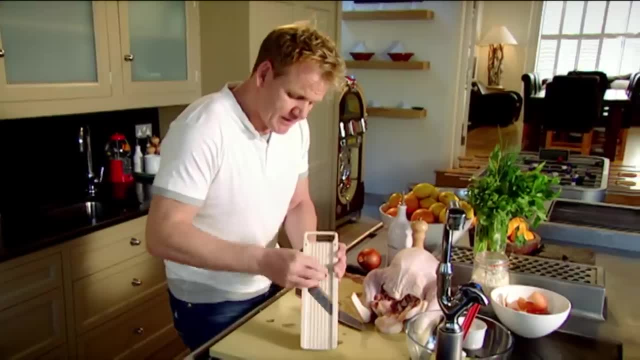 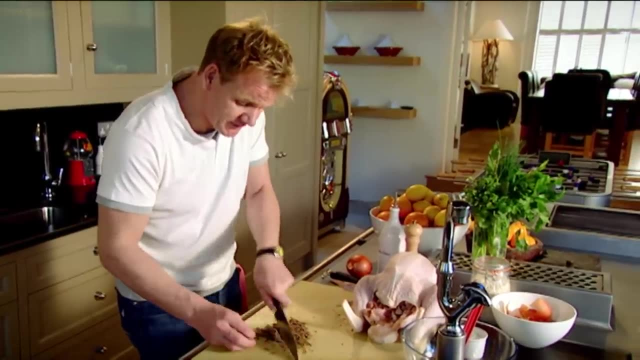 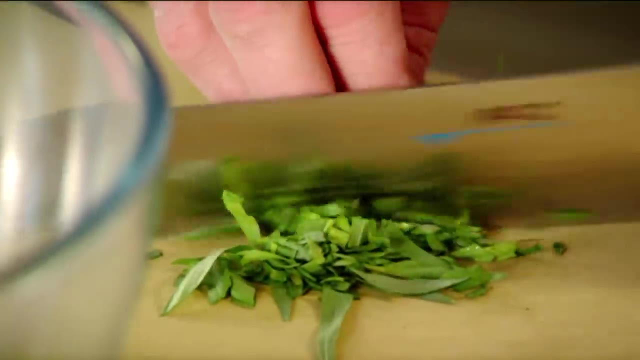 Yes, it's expensive, but boy, is it worth it. Don't chop the truffle too small, because we want to taste and identify the truffle. Parsley, Tarragon, Salt, Touch of pepper, Tablespoon of olive oil. 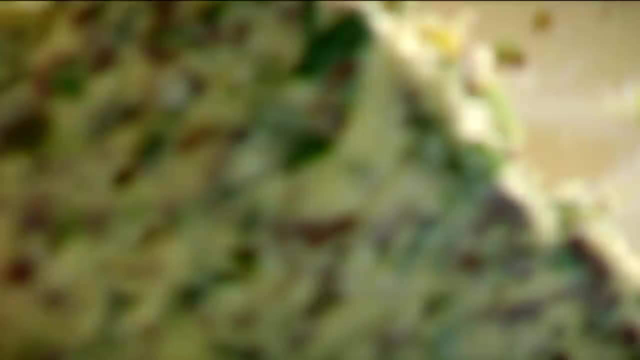 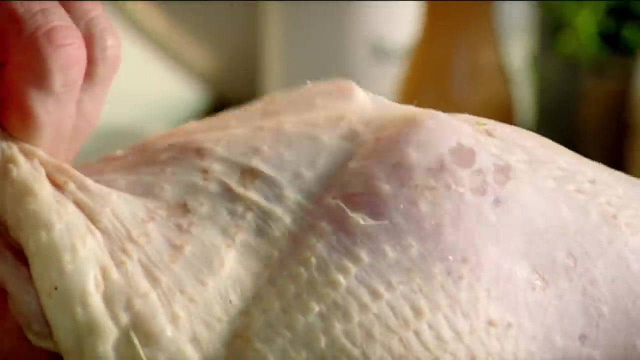 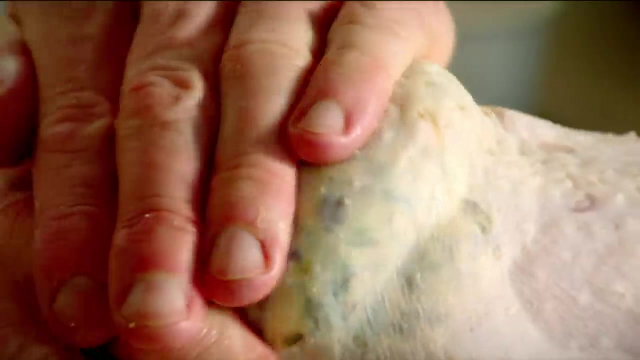 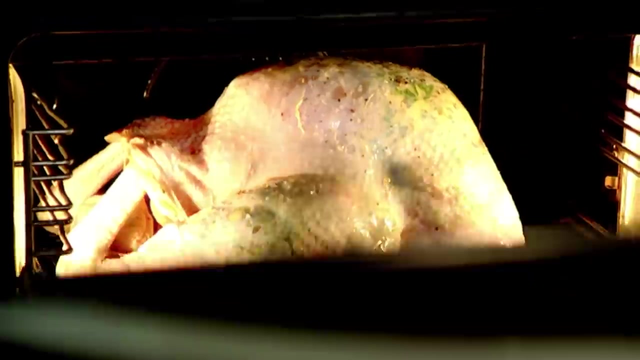 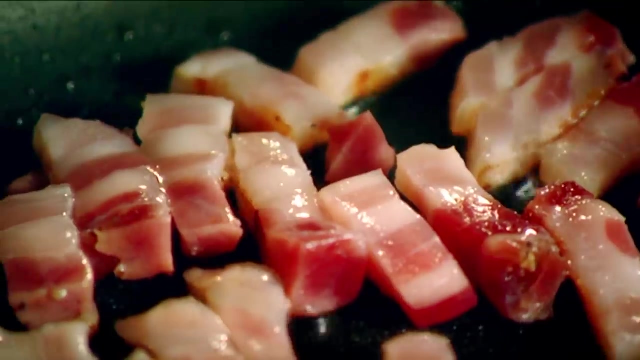 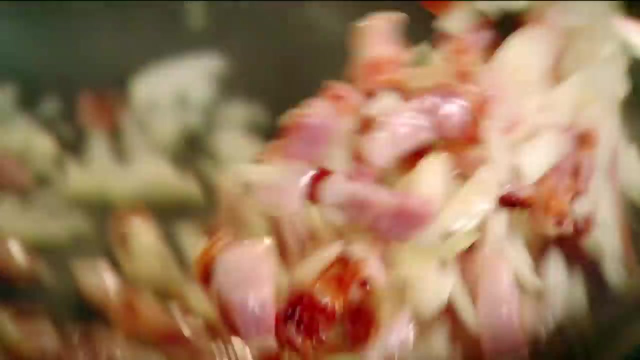 And that stops the butter from burning. Take your piping bag and fill it. Separate skin from meat. Piping bag in Pipe butter. Massage Salt, Pepper, Olive oil, Roast, Citrus, breadcrumbs, Pancetta, Onion, Thyme. 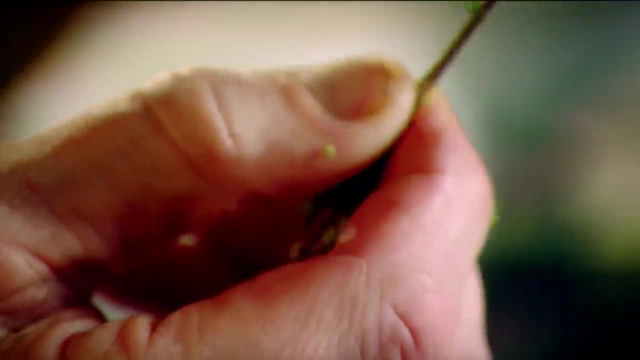 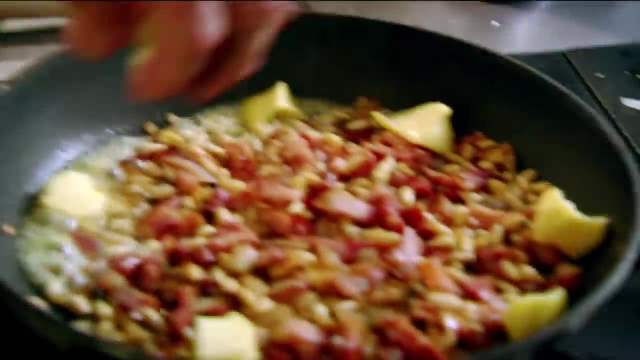 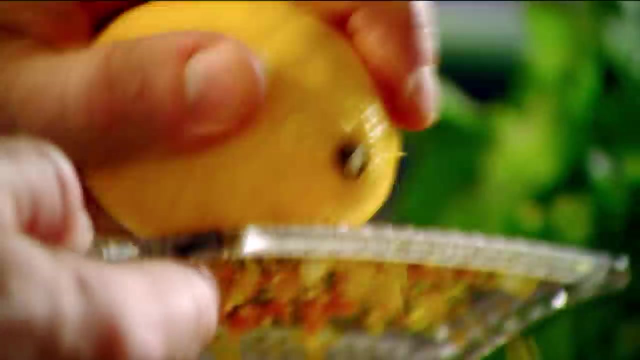 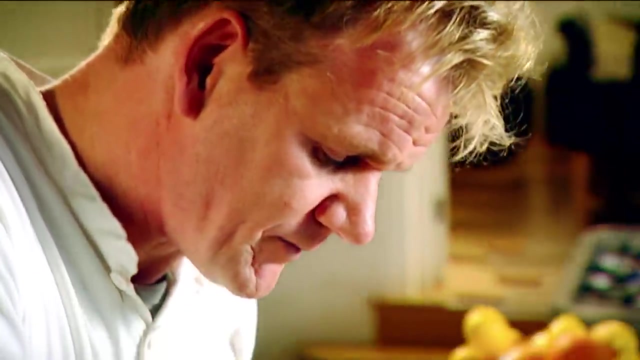 You don't need to do a good old chef's trick and pull down and just peel it off his lovely flowers: Pine nuts, Butter Bread, Orange, Lemon. As it starts browning, sprinkle the orange and lemon breadcrumbs. Lemon juice.